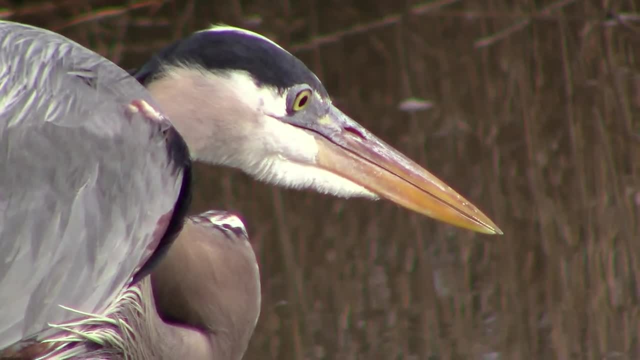 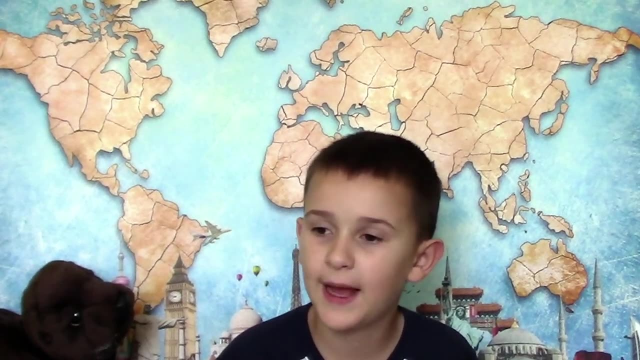 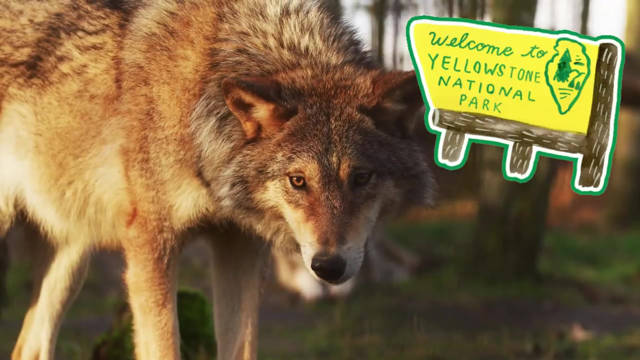 and each other to survive. If you take one plant or animal out or change the climate, it affects the entire circle of life. My favorite extinct animal ever is the passenger pigeon. The passenger pigeon went extinct because it was over hunted. One example would be the wolves of Yellowstone Park. Due to hunting, they almost became extinct. 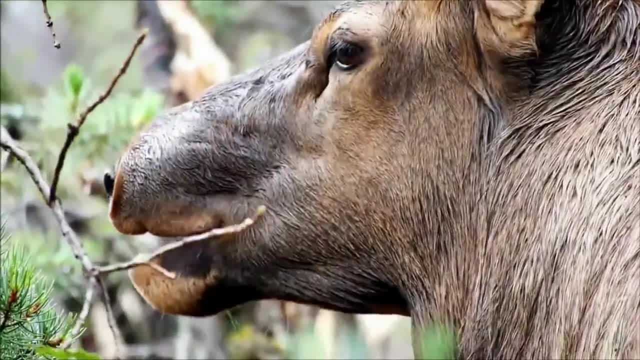 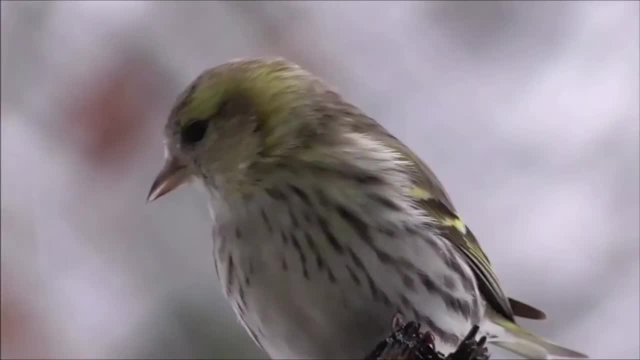 in 1930.. Without them, the elk and the deer that they preyed upon thrived, but their overgrazing of plants destroyed the streamside willows in Aspen, which were the habitat for the cute songbirds. Without the willows in Aspen, the river started to erode, taking dirt from the riverbanks. 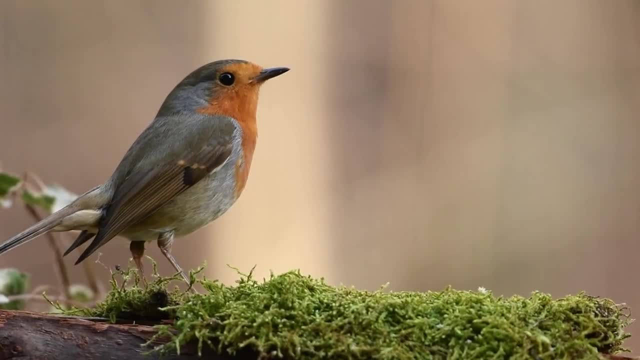 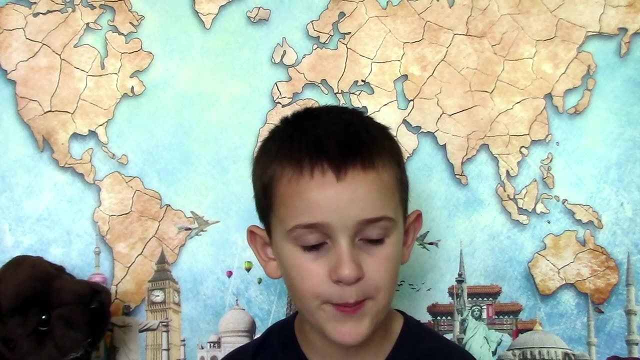 The loss of the songbirds and other animals in the river started to be a problem. The songbirds and other birds that eat bugs led there to be more mosquitoes and other insects. Mosquitoes bug me because they just drink my blood and they bite me too much. 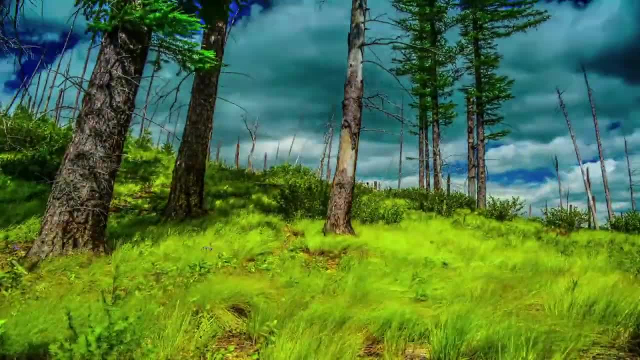 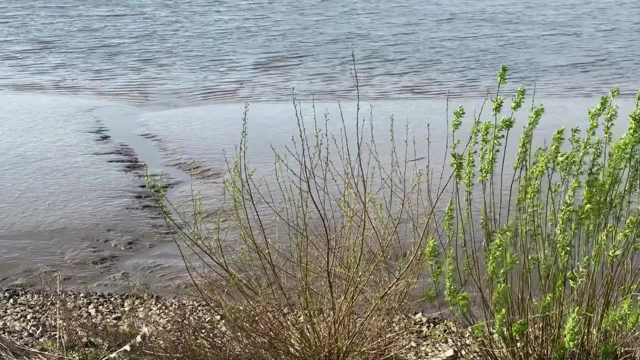 So without the wolf the entire ecosystem was out of balance. When the wolves were brought back to Yellowstone Park in 1995, they did prey on the elk and the deer, but plant life returned to the riverbanks and many animals returned, including birds. 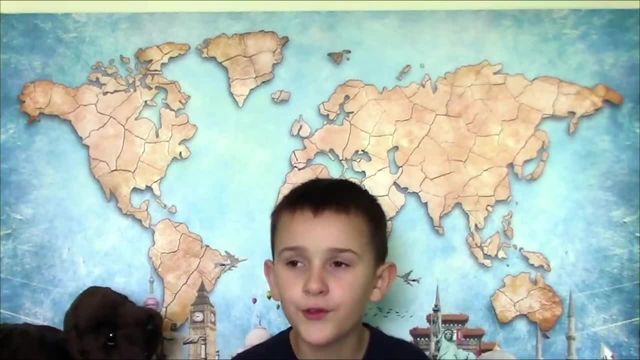 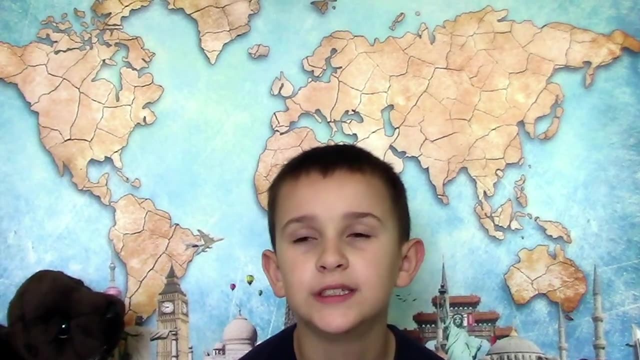 beavers, fish and other animals. If you take one animal out of the riverbanks, you can see that the riverbanks are full of animals. If you take one plant or animal out, it messes everything up. You mess up the whole ecosystem. 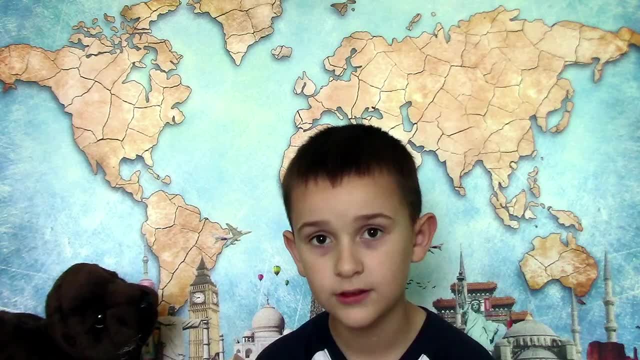 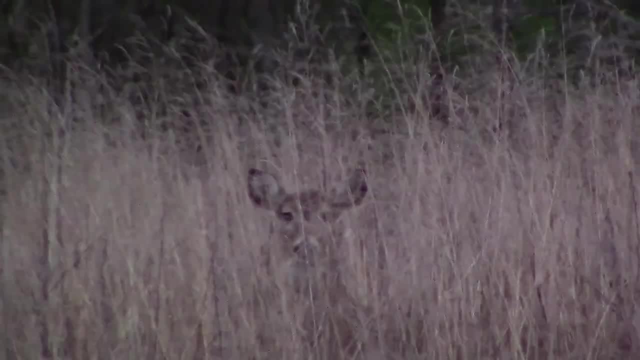 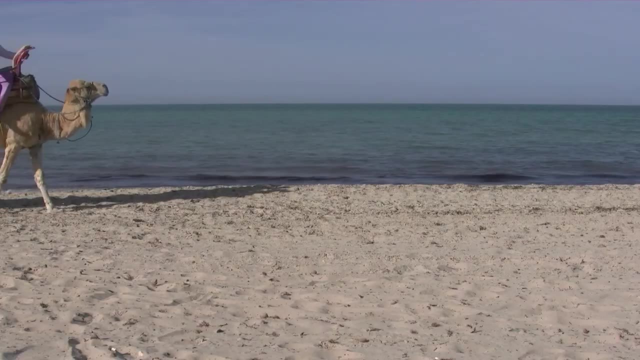 If you take the villagers out of Minecraft, zombies will have nothing to eat. Plants and animals evolve over time to survive in the habitat they live in. An example would be camels, who were built to survive living in a desert. They can travel up to 100 miles without taking a drink of water. 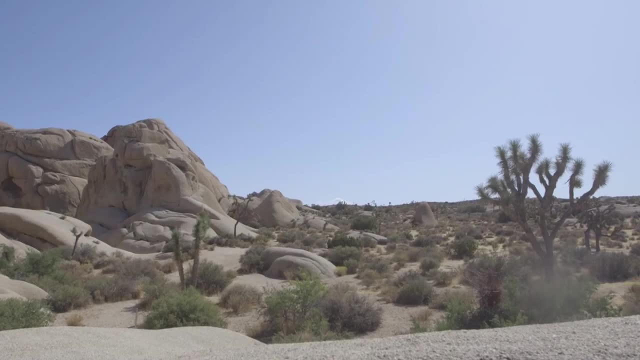 Camels can get water by eating the desert plants, such as cactus and other plants. They can also eat the water of the desert plants. They can eat the water of the desert plants, such as cactus, when they need to hydrate. 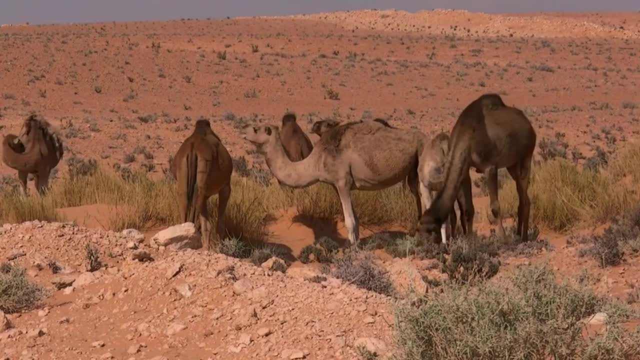 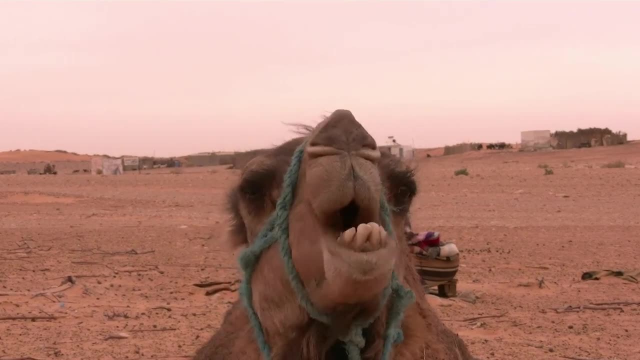 For extra long trips. they can use fat reserves on their humps that can be broken down in the food and water when they need it. They can also close their nose and eyes to keep out the sand. For all the great ways they can adapt, they would not be able to adapt in the cold of. 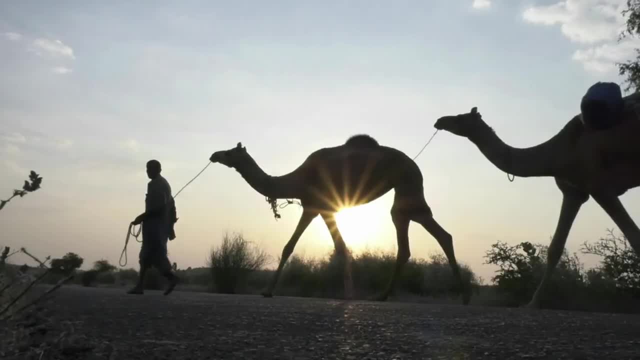 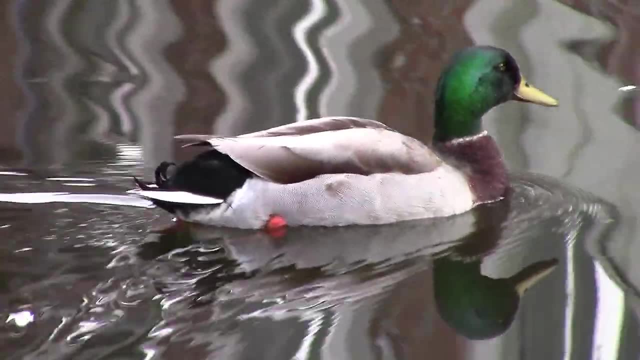 Antarctica. Their strengths to adapt would not help them Because their bodies are not used to the cold, they likely wouldn't survive. What animals live in your habitat and why are they important? Thank you for watching. Please like and subscribe.